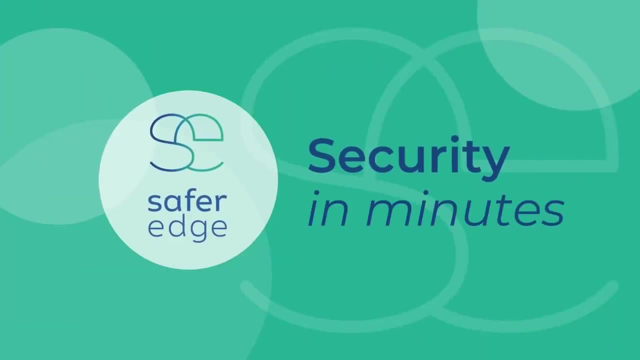 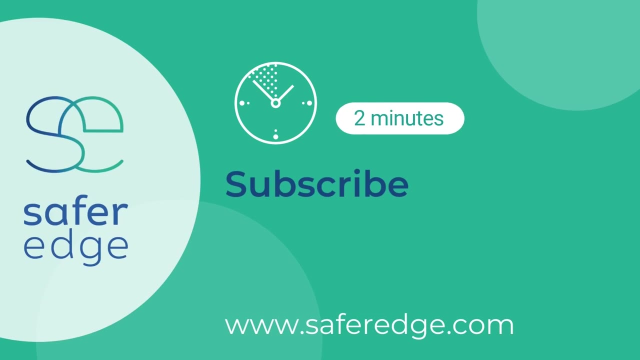 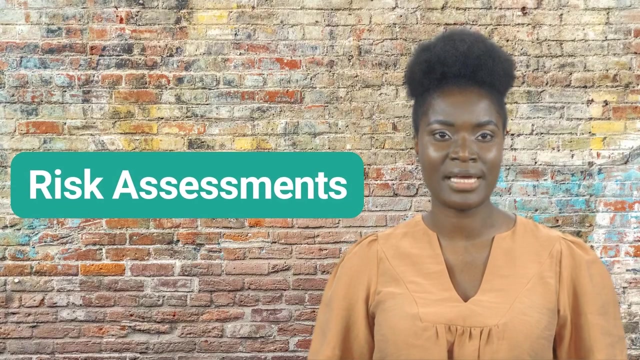 Welcome to Security In Minutes, a microlearning series from Safer Edge where we introduce or explain a security topic in two minutes. Click subscribe to get a new microlearning in your feed each week. Today, we learn about risk assessments. Everyone assesses risk every day. It's how we keep ourselves. 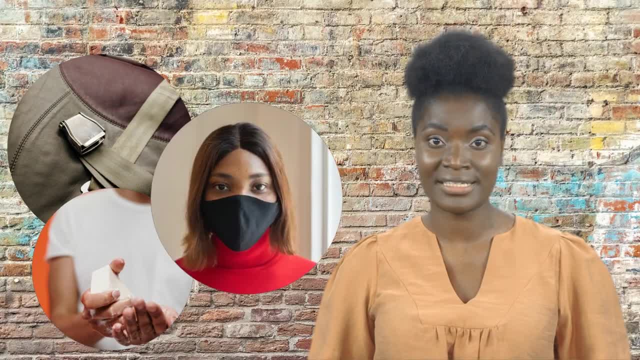 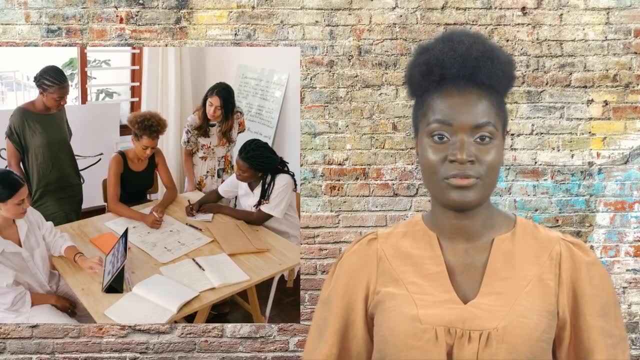 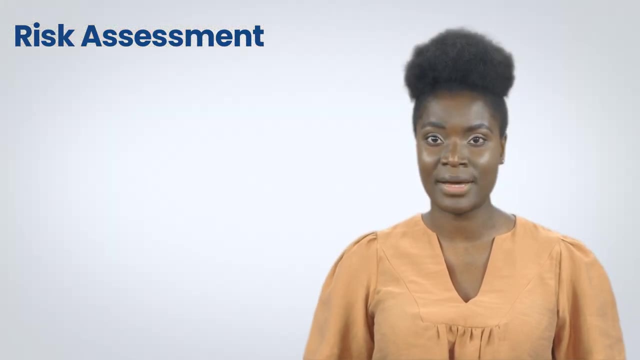 safe and alive. We look for dangers around us and then apply safety measures. Organizations are required to assess the risks they create for the people who work for them. This process is called a risk assessment. While there are many different formats for a risk assessment, all of them contain at least three basic steps. Step one: identify threats. 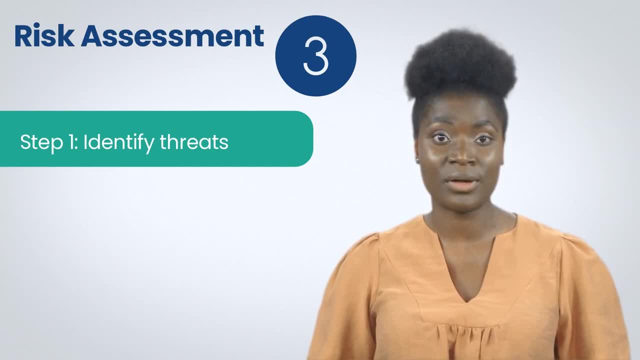 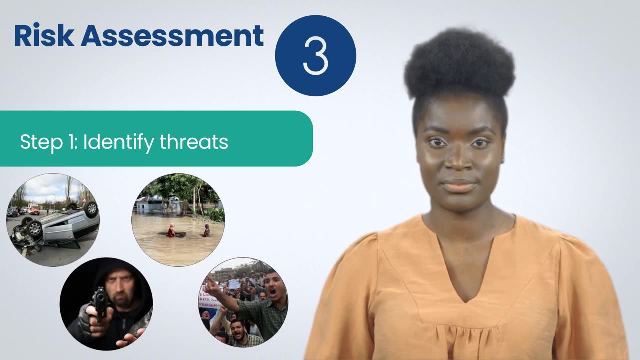 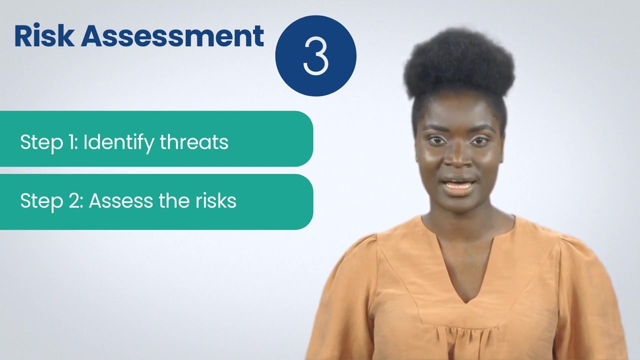 Threats are any danger or hazard that you will face in your work. Threats may be accidents, crimes, natural disasters or people opposing the work you do. Step two: assess the risks. You need to know how dangerous something is And you find this out by 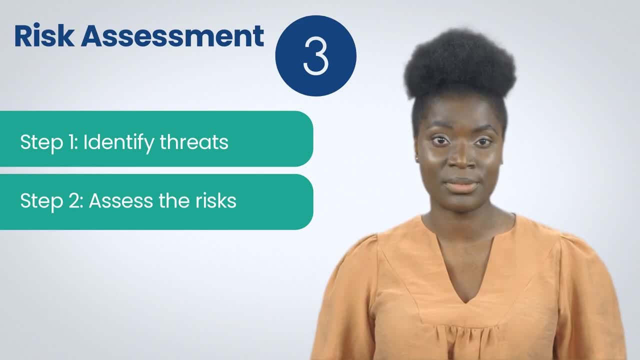 evaluating how likely a danger is and what the impact would be if it were to occur. Some threats will be likely and dangerous. some will be minor. To decide whether a threat is high, medium or low, you can download the risk metrics template below. 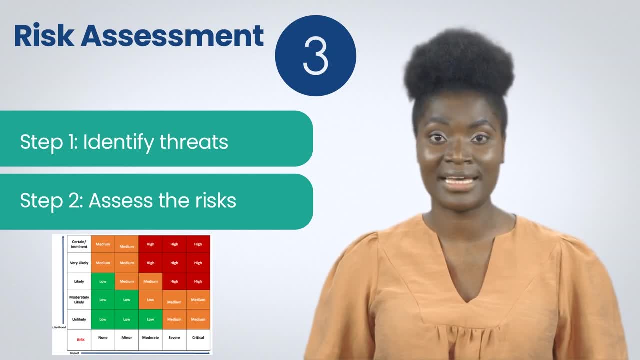 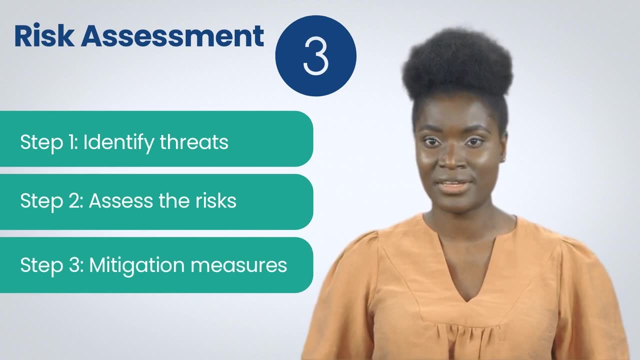 Simply move each threat along each axis, based on likelihood and impact, to get a risk rating. Step three: mitigation measures. To work safely, we must reduce the likelihood of hazards or their impact. These are mitigation or safety measures. For example, we could train drivers to avoid car. 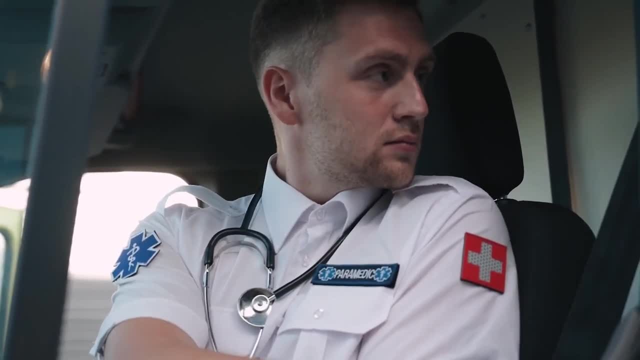 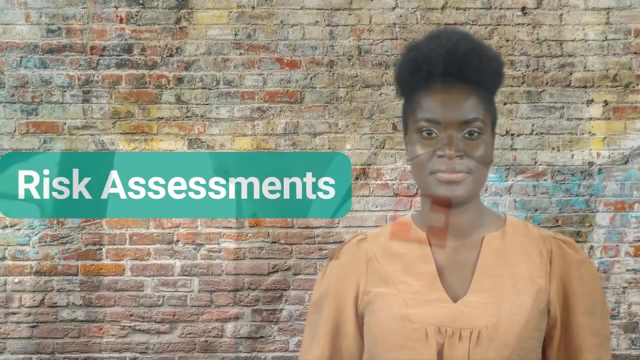 accidents. We could require seatbelts to lessen accident damage. Safe driver training and seatbelt use are important. We need to know how to avoid car accidents. We need to know how to avoid car accidents. Use our mitigation measures. And that is risk assessment in three simple steps. 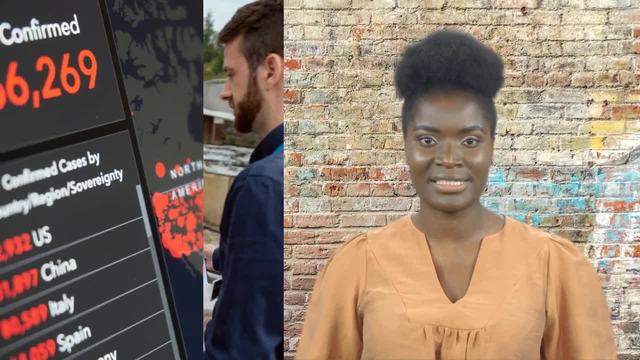 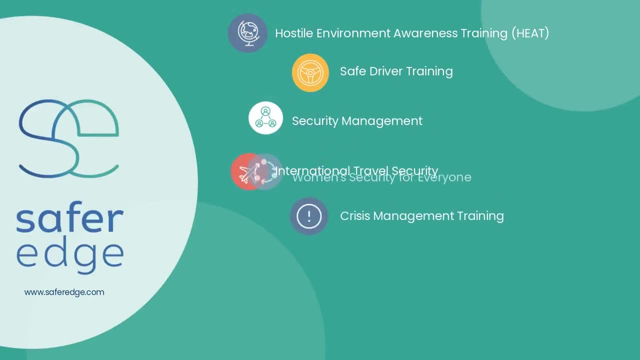 You can practice risk assessment by thinking about the risks you face in your everyday work. Safer Edge provides engaging, affordable, on-demand e-learning in multiple languages that can be customized to your organization. Send us an email to learn more.